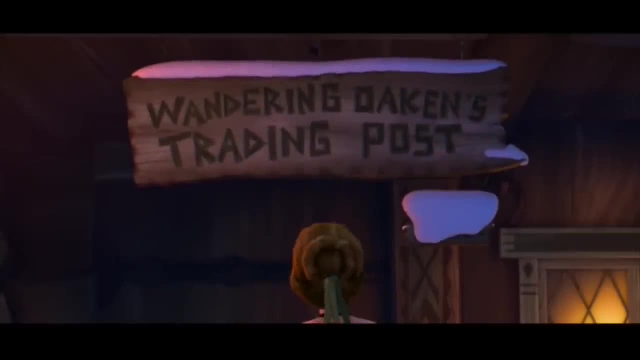 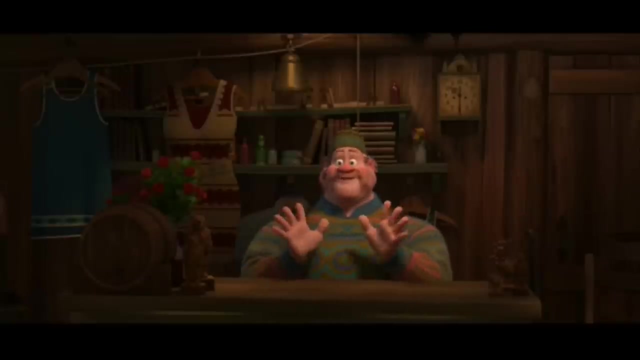 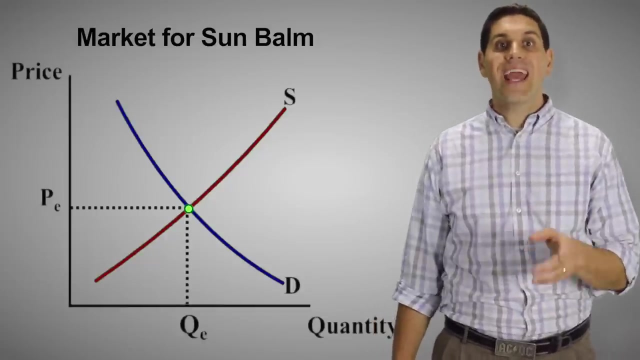 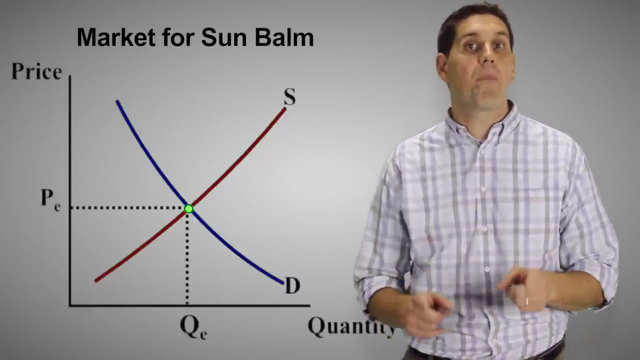 In this scene, Princess Anna walks into Wandering Oaken's trading post and we find out what happens when there's a change in a market. Using this example from Frozen, let's analyze the market for a sun balm. The point of learning supply and demand is to understand what happens to price or quantity when there's going to be a change in a market. 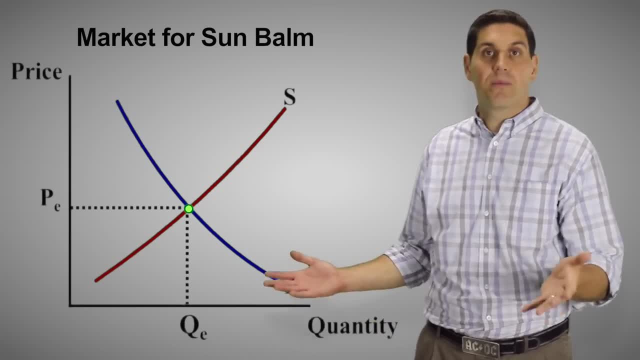 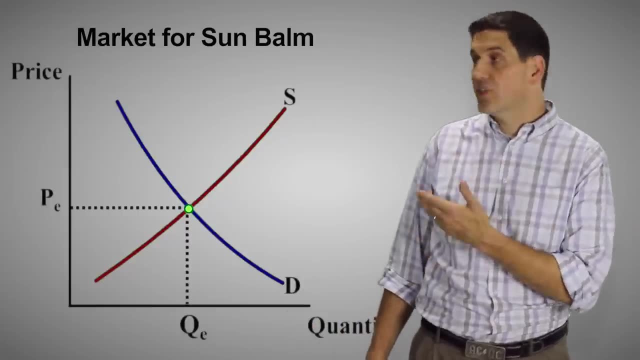 So this graph helps us to predict what happens when we find out there's going to be a change. The change that happens is that summer suddenly becomes winter. So what's going to happen to the supply or the demand for a sun balm? Well, it's definitely going to affect demand because it's going to affect consumers. 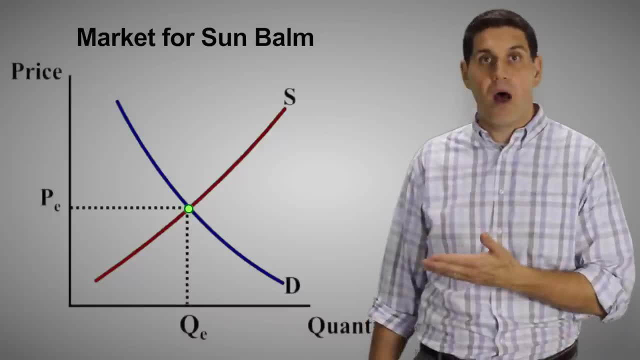 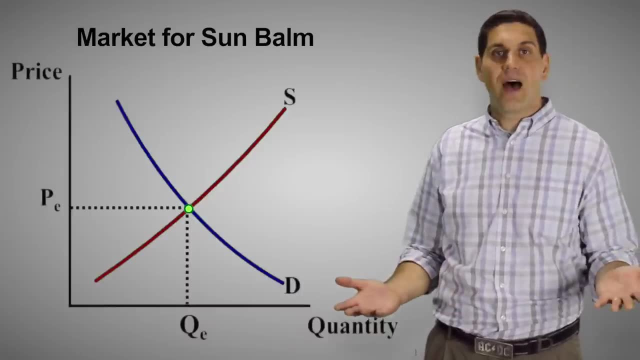 It's going to have no effect on supply or the production of sun balm. Now, is the demand going to go up or is it going to go down? Well, of course the demand is going to go down because people don't want to wear sun balm during the wintertime. 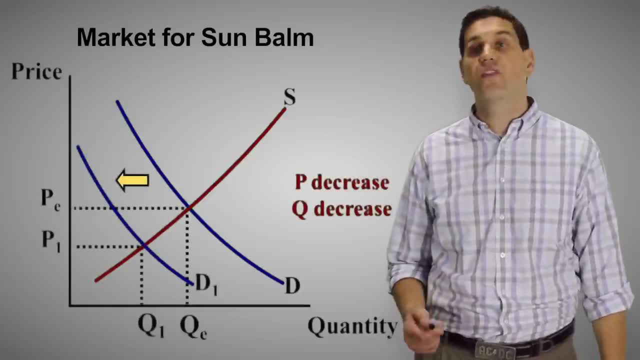 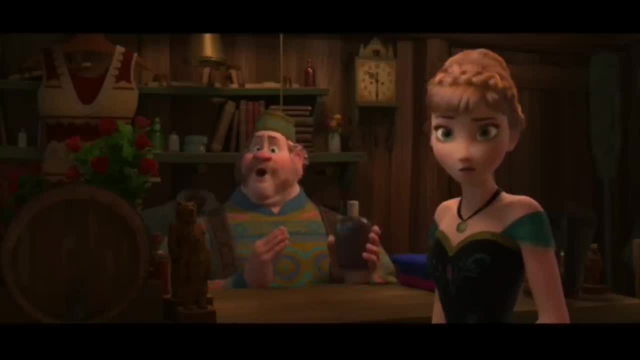 They want to wear it during the summertime. So the demand is going to decrease or shift to the left. The new equilibrium is right here, And so the price and the quantity is going to fall. Woohoo, Big summer blowout. 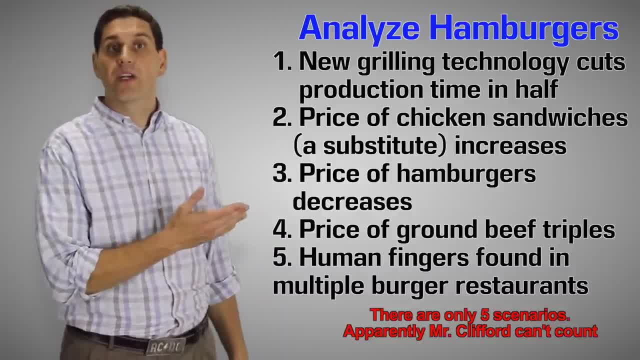 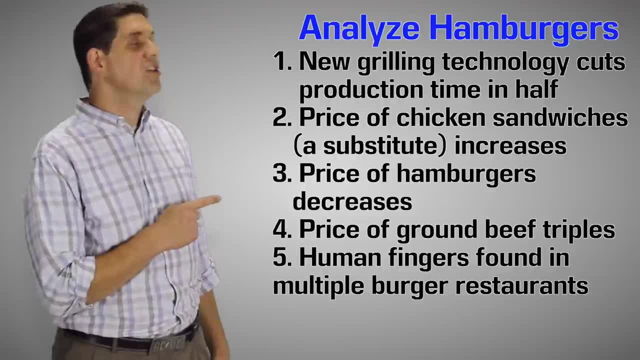 Now it's time for you to practice. I have six scenarios right here for hamburgers. Your job is to figure out if it's going to be an increase or a decrease in demand or supply, what shifter it is and what happens to price and quantity for each scenario. 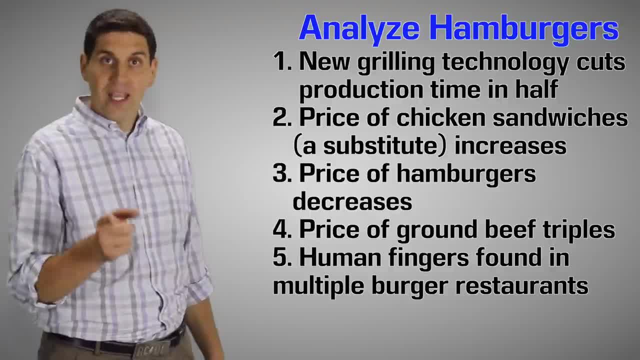 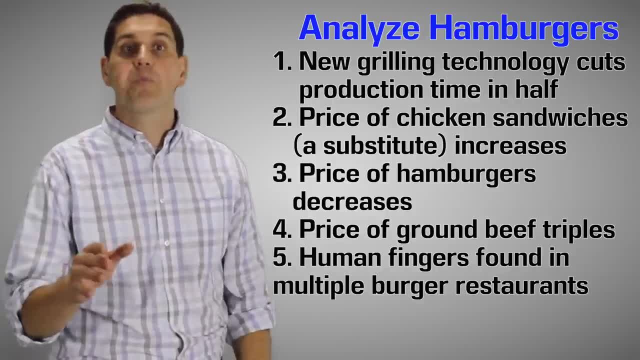 So get a piece of paper and draw six supply and demand graphs and show on each graph what happens for each one of these scenarios. And remember, for each one of these things we're analyzing hamburgers. Make sure to pause the video and then I'll explain each one, all right. 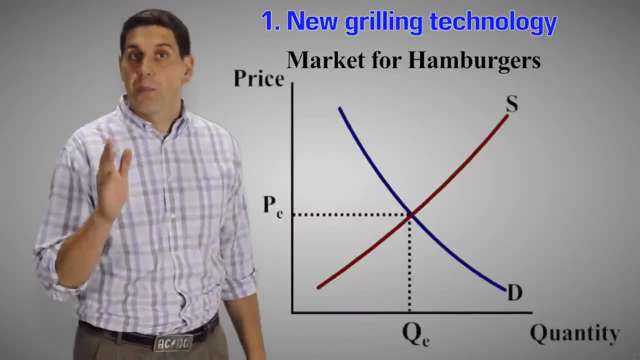 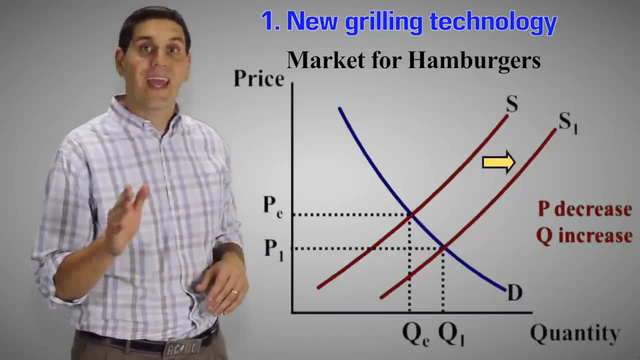 Good luck For the first one. new grilling technology would cause a supply to shift to the right or increase. Now this is supply, because this is something that's going to increase the production of hamburgers. And remember, technology is a shifter. 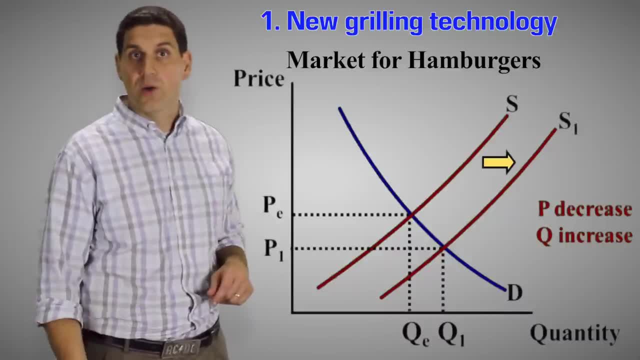 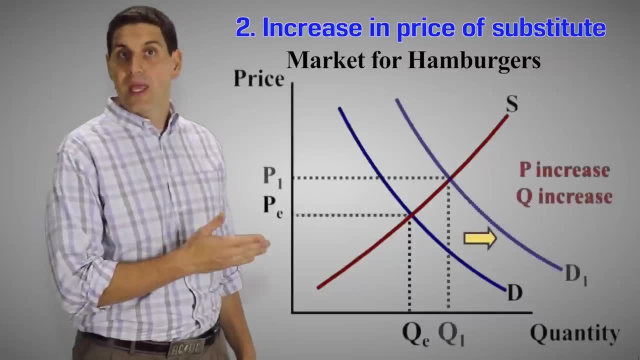 The graph tells us the price will decrease and the quantity is going to increase. For number two, an increase in the price of chicken sandwiches- a substitute- is going to cause the demand for hamburgers to increase. Remember, the price of related goods, substitutes and compliments- is a shifter of demand. 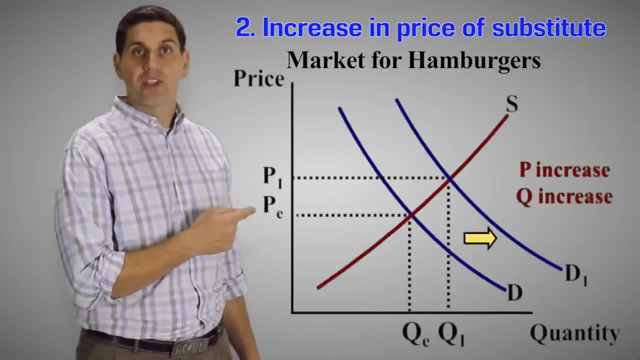 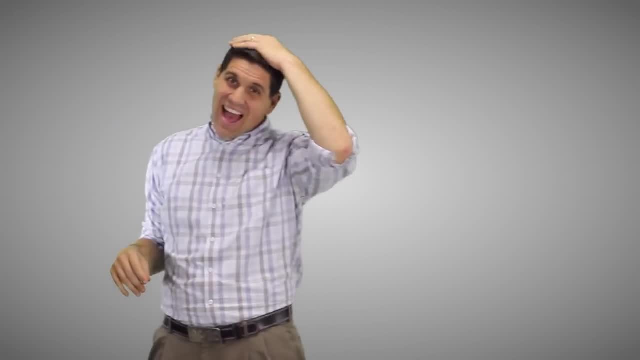 And if chicken sandwiches are more expensive, that means people are going to buy more hamburgers. So the demand for hamburgers shifts to the right. So price increases. Price goes up and quantity goes up. Ah, one rug hair bro, Ah nah. 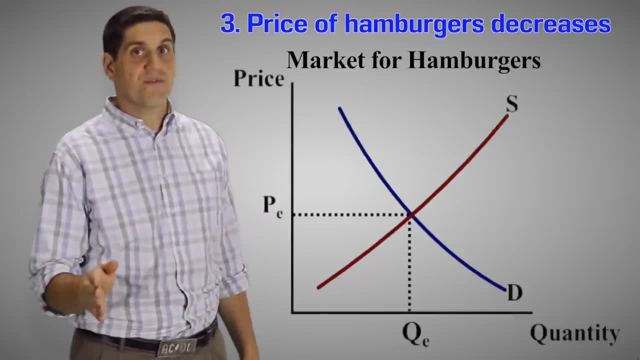 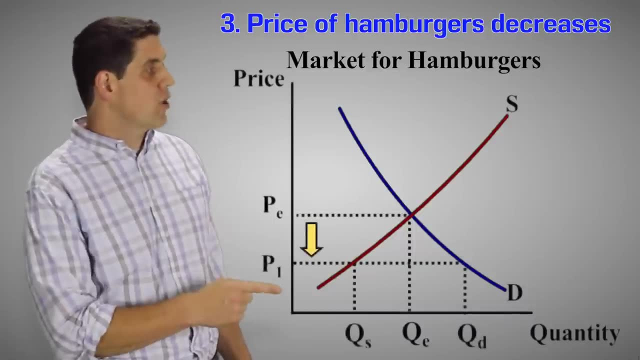 For number three, if the price of hamburgers decreases, that's not going to shift the curve. Remember, a change in price does not shift the curve, It moves along the curve. So if the price goes down, the quantity of demand is going to increase. 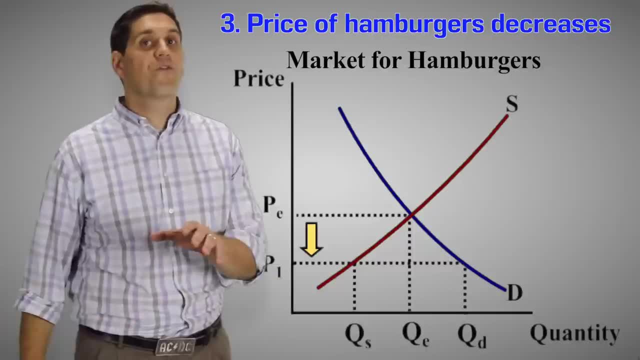 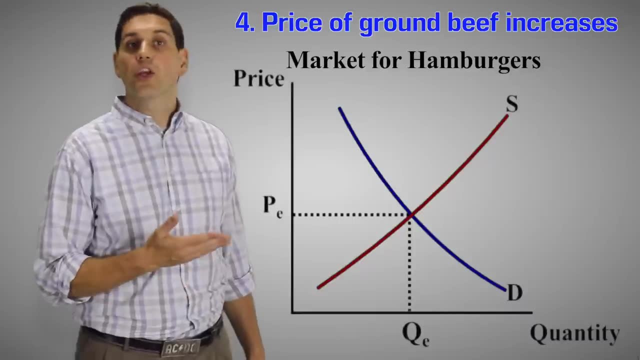 The quantity supplied is going to decrease and that's going to lead to a shortage. Don't forget: price never shifts the curve. For number four: if the price of ground beef- a key resource in the production of hamburgers- increases, that means we're going to produce less. 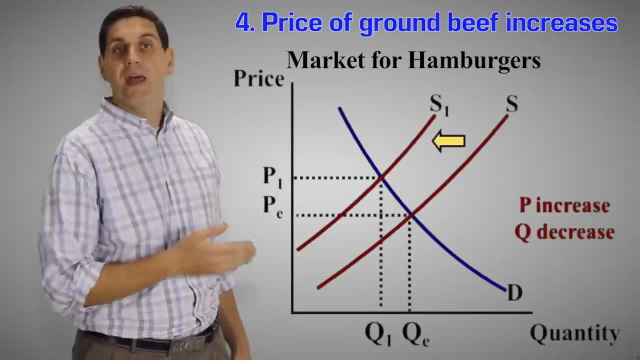 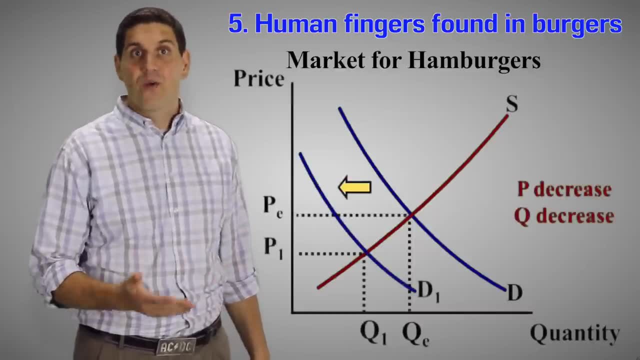 hamburgers. So the supply will shift to the left, price will go up and quantity will go down. And for the last one, if there's human fingers found in many restaurants, that's going to decrease the demand for hamburgers, right. 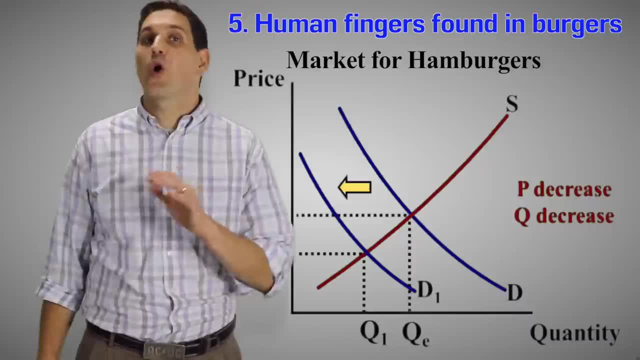 So the demand shifts to the left, price goes down and quantity goes down. So a real quick story. One time I was doing that example in class and I had a student who said that it wasn't going to be demand, It was going to be a supply shifter. 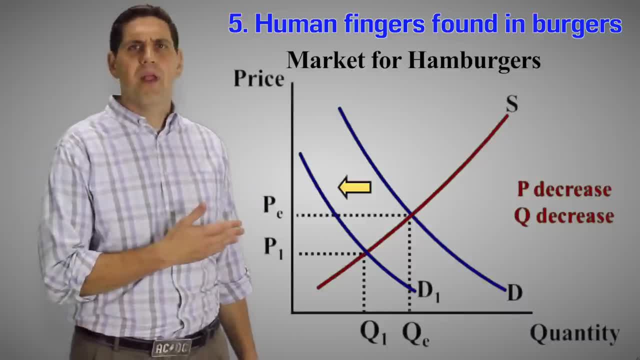 The supply would go down. So I walked up to him and I said: well, why do you think it's going to be a supply shifter, not a demand shifter? And this innocent student says: well, if your workers don't have any fingers, then now you're going to have to go to the grocery store. 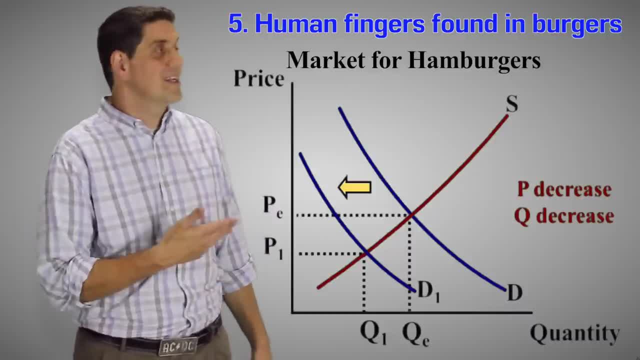 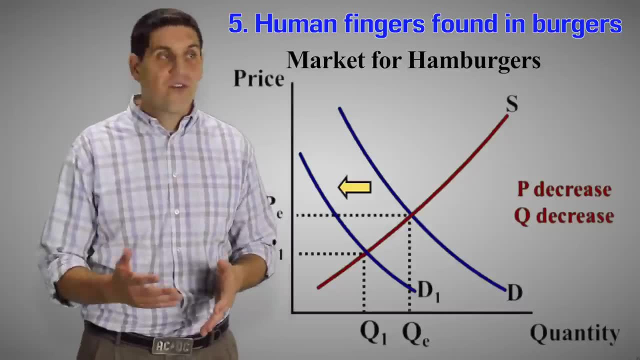 If your workers don't have any fingers, then that means they can't produce as much, and so that's going to decrease supply. Well, it's definitely going to be a demand shifter. If there's fingers found in food, people aren't going to buy it. demand's going to decrease. 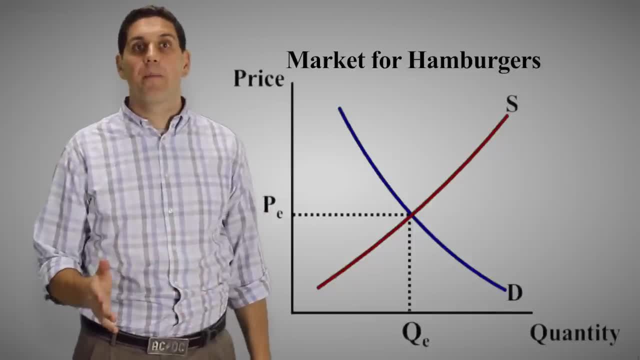 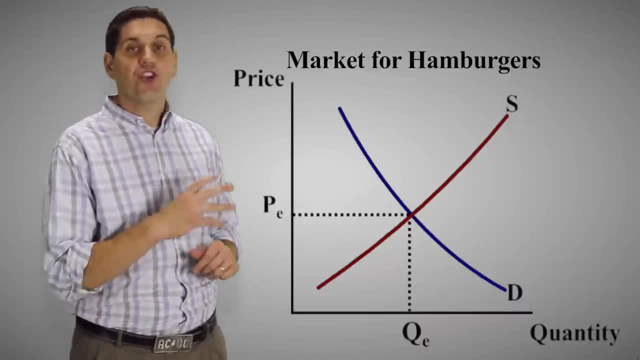 Now, whether you're in high school or college, you're taking microeconomics or macroeconomics- it's super important to understand supply and demand. Understanding this graph is not just good for class, it's also good for life. You can predict changes in the market. 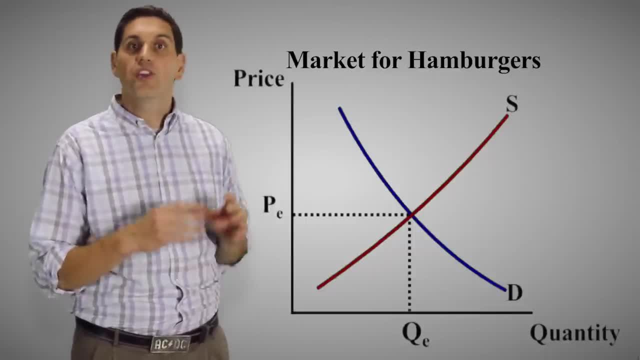 It can help you if you're in business or if you're a consumer buying things, because you know what's going to happen. So you're going to have to go to the grocery store. So you're going to have to go to the grocery store. 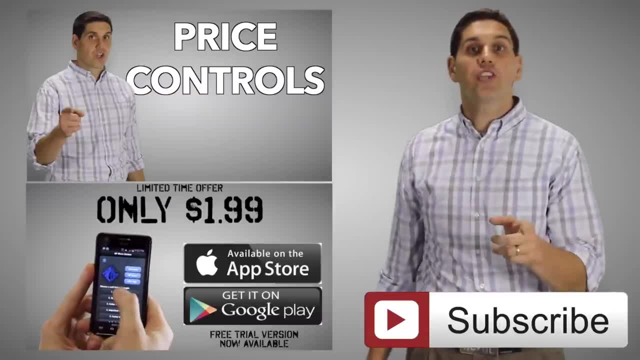 So you're going to have to go to the grocery store Now. I hope this video was helpful. Now, I hope this video was helpful. Make sure to take a look at the next video that's going to explain price control, something called price ceilings and price floors. 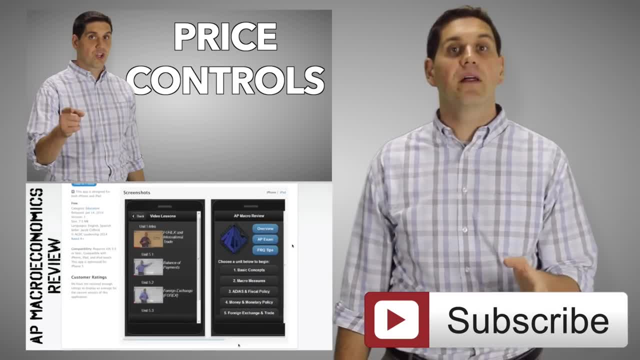 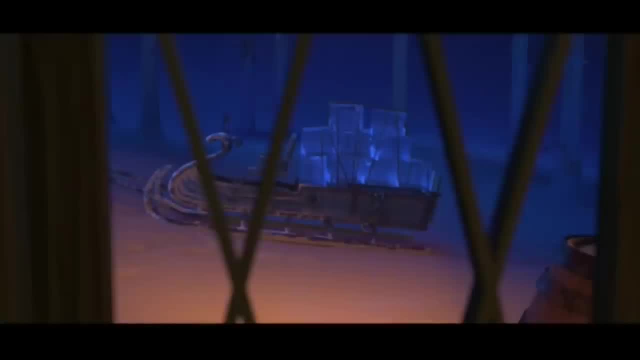 and take a look at my review app for your smart phone or tablet so you can get ready for the next test. All right, Until next time You want to talk about a supply and demand problem, I sell ice for a living. Ooh, that's a rough business to be in right now. 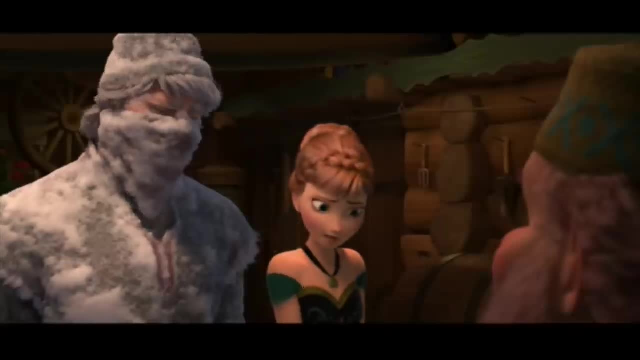 I mean, that is really, That's unfortunate.